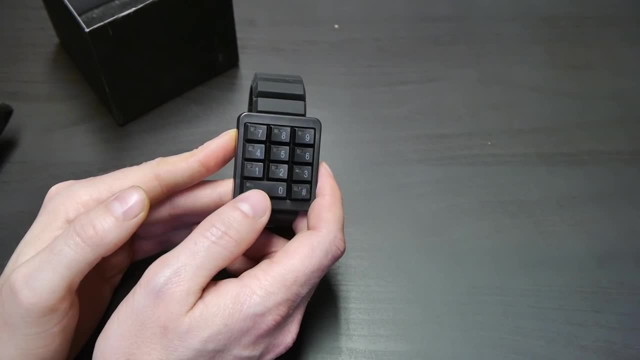 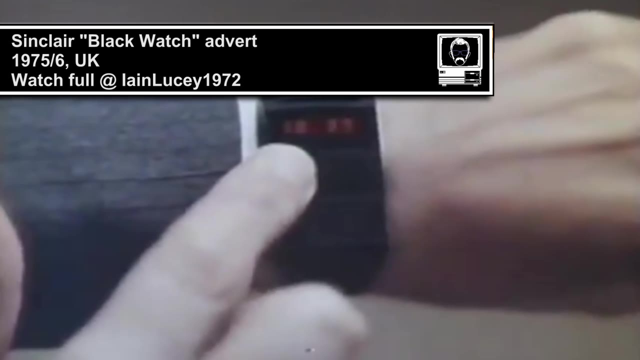 The watch operates by pressing a button, which then reveals the time on one digit after another, reminiscent of the Sinclair Black watch that used a button to activate in order to save battery life. Waddupe buddy offen. Open home expectations horny, dishonest. 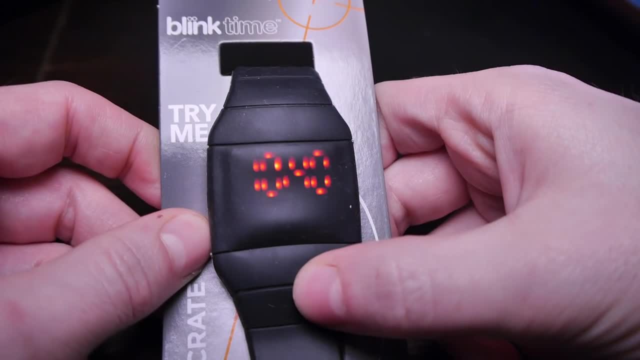 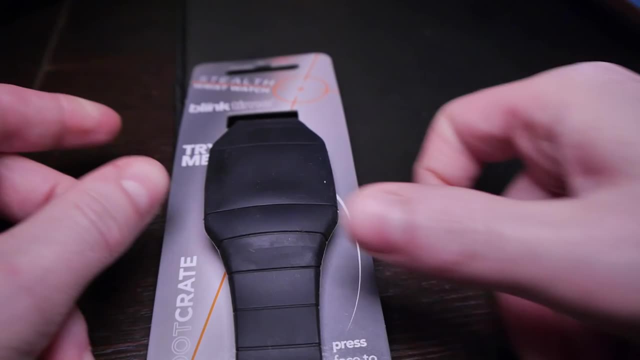 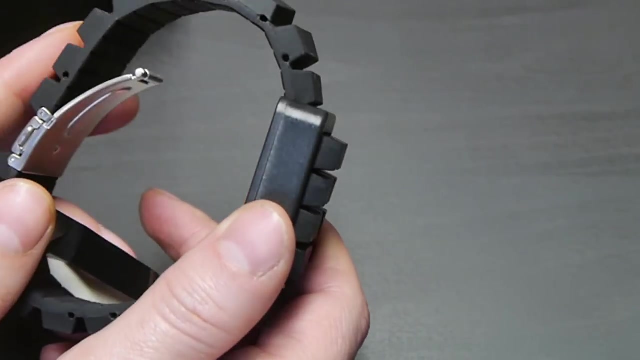 A modern day version, here known as the Stealth Watch, which is really a bit pointless. I suppose it stops other people from copying your time. but even without the keyboard this thing has retro heritage. It also reminds me of those awesome Casio calculator watches, but of course this doesn't. 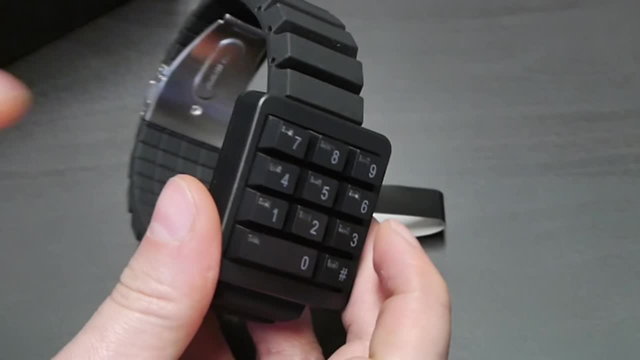 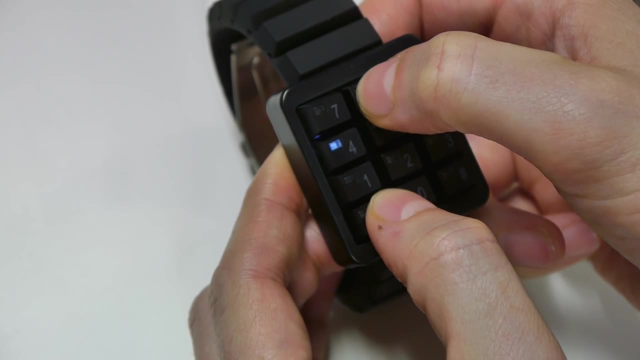 actually calculate anything other than how much of a sucker you are for buying it. You can change between 24 and 12 hour modes by holding 0 and 8 for 2 seconds. The watch will then display either 24 or 12 to indicate the current mode. 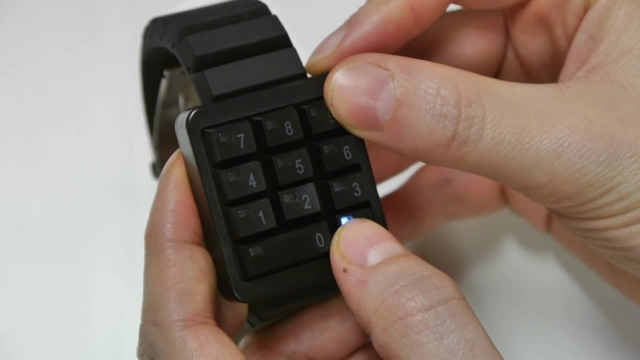 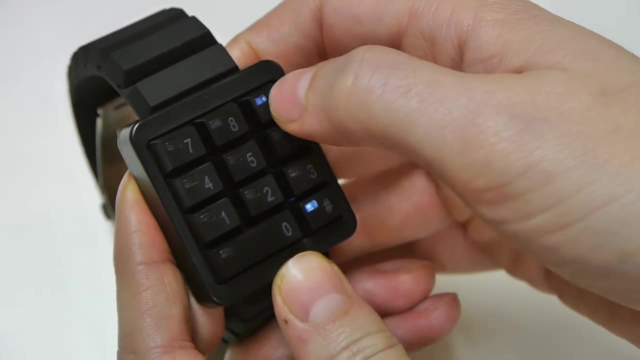 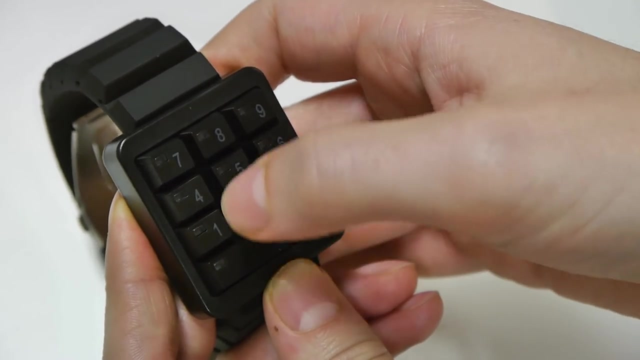 Setting the time then involves depressing hash and 9 for the same amount of time. You can then jab the time in as it's written, so 20.09 will be 20.09.. You can then set the date by using the American system of entering the month first. 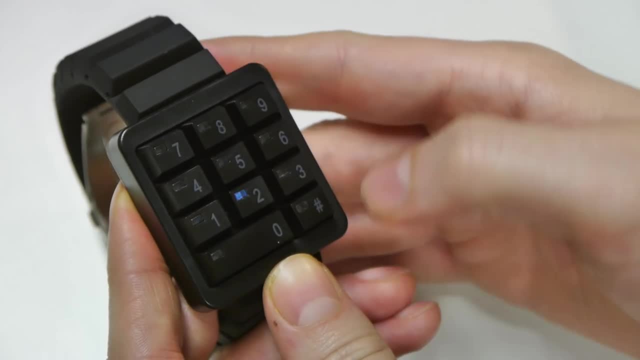 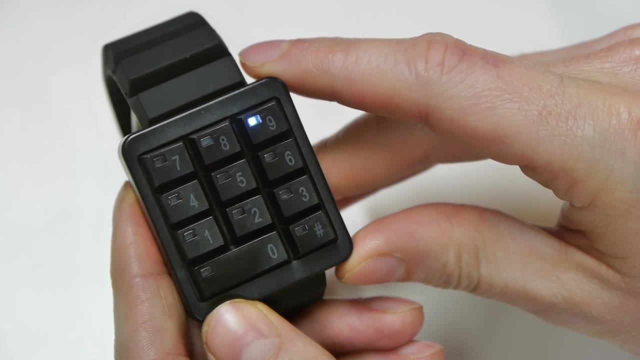 So 04 for April and 07 for the day. Then job done. To display the time, You can press any key other than hash, whilst hash will give you the date. Other than that, the watch has no further functions well, other than to give you that. 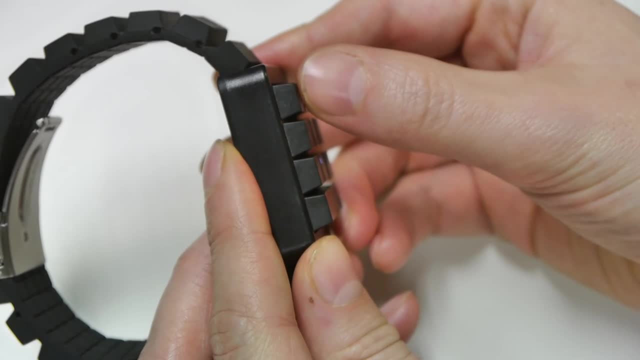 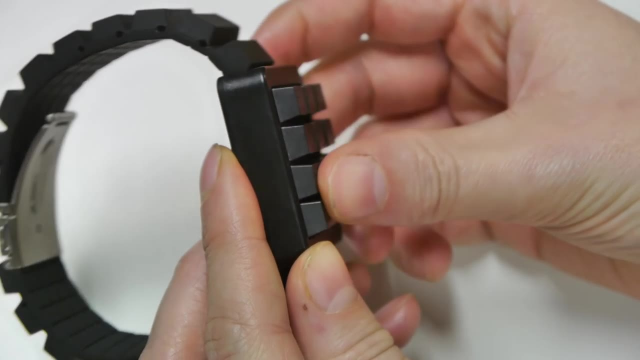 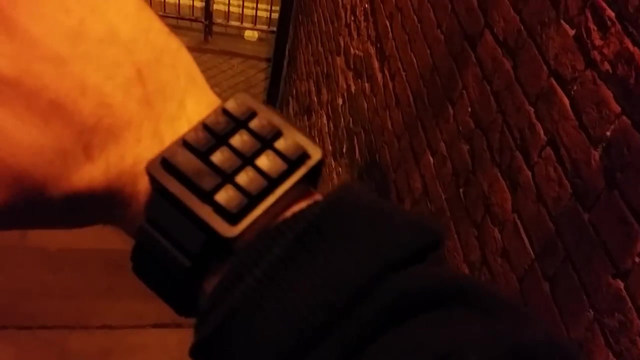 satisfying urge to press a computer key. It's not as clicky as I'd hoped- there's no clicky mechanical switches here, I'm afraid- but it still feels warming and a little pleasing to have access to keys on demand, Particularly when you're outside venturing in the scary real world and you just need 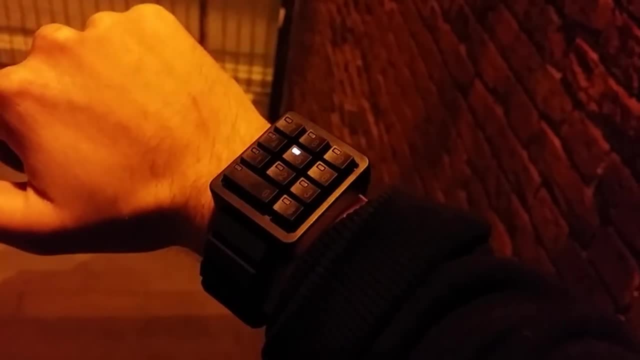 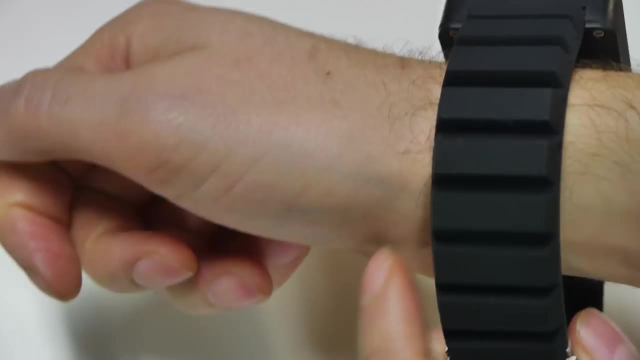 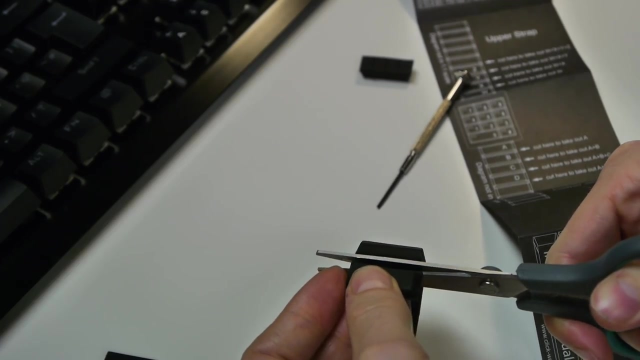 the comfortable reassurance of a numeric keypad to guide you home. Don't worry, Microsoft Excel is just around the corner. Of course, before you get to that stage, there are a few issues to address, The first being the strap size. Thankfully, you can just snip the strap down and achieve a snug fit. 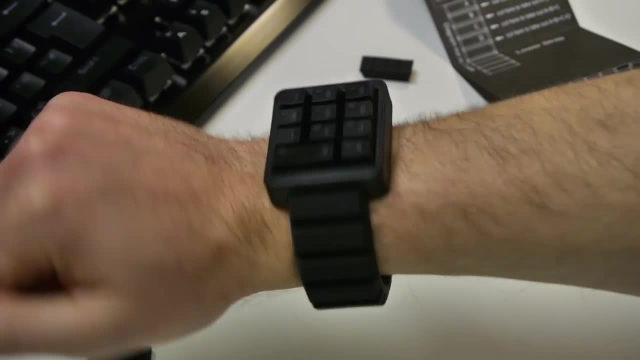 Of course, this means that, should you wish to sell on the watch, anyone with larger wrists than you is in for a tough time. This limits your sale market to people of ever decreasing size. I'm not sure if that's a good thing or not.